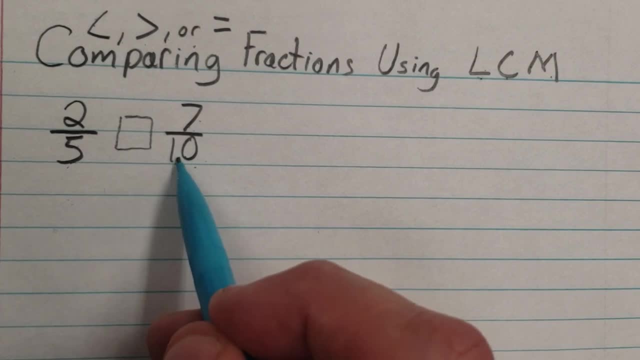 Since our denominators are not the same, we are going to have to use the LCM least common multiple to make them the same. If the bottom numbers denominators were the same, then we can also get the tops to decide which one has a greater value. 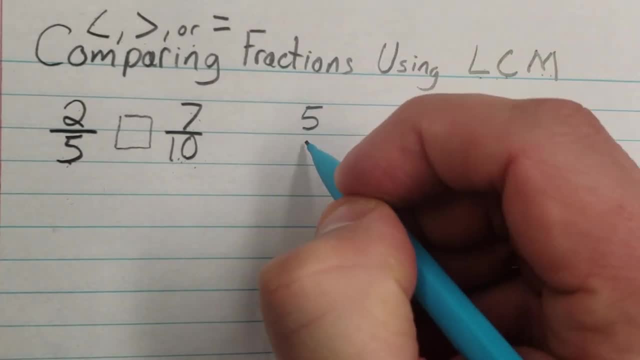 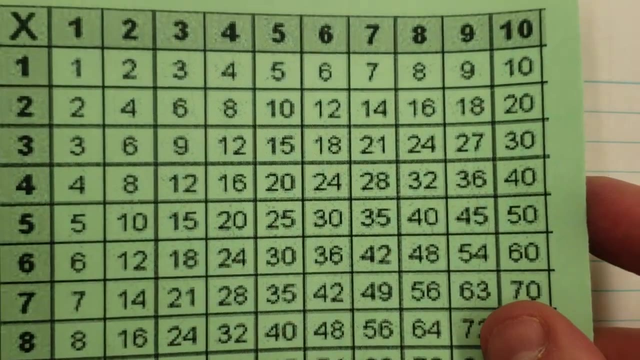 So 5 and 10 are different, so we need to find the LCM of 5 and 10.. In order to do that, we're going to skip, count or use a multiplication chart to help us with that. We need our 5ths and we need our 10ths. 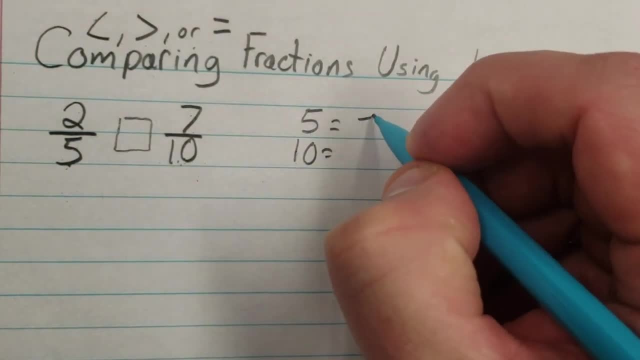 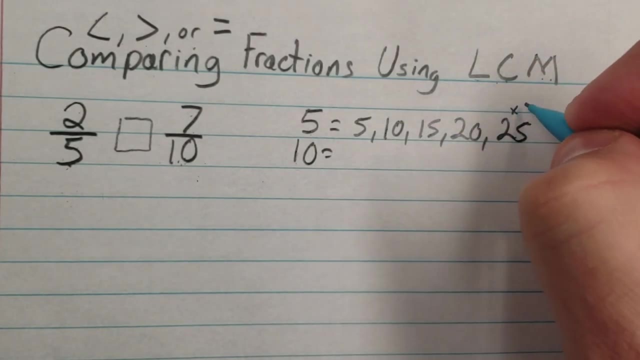 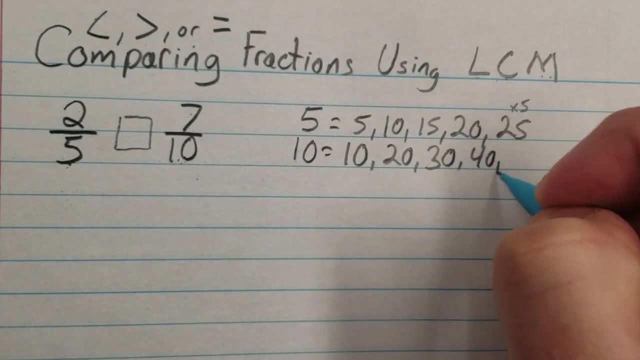 So for our 5ths, we're going to go until we get the times 5., 5,, 10.. 15,, 20, and 25.. That brings us up to 5 times 5., 10,, 20,, 30,, 40, and 50.. 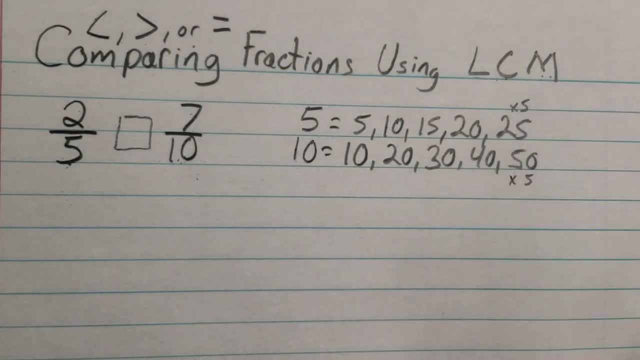 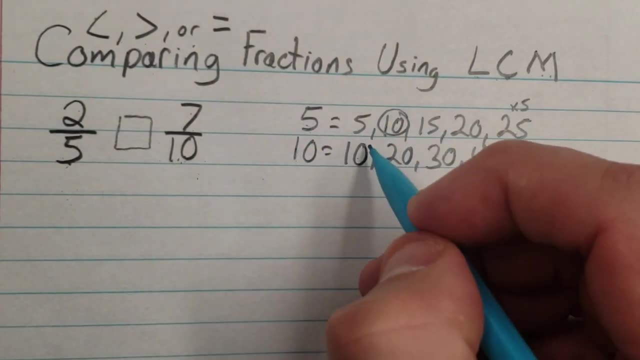 That brings us up to 10 times 5.. Those are our multiples. Now we need to find what they have in common. That means the same 10 has a 10 on it, and so does 5.. Notice they both have a 20, but 20 would not be the least. 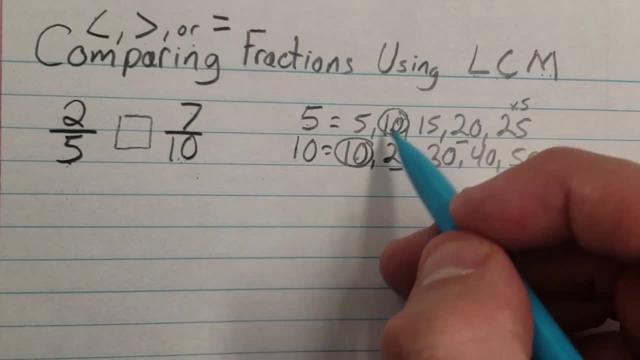 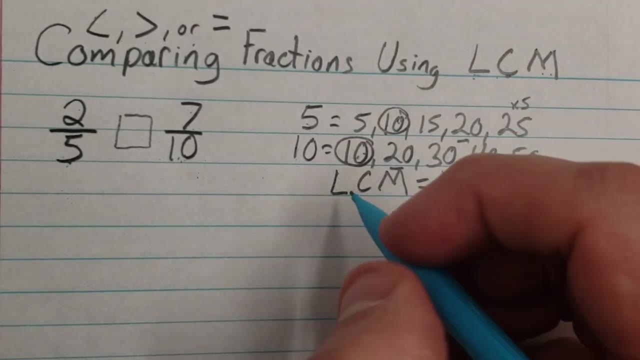 Least means the smallest. The smallest is the littlest number. They both have a 10, and that's the littlest one. So 10 is our LCM. What are we going to do with our LCM? It's going to become our new denominator for both fractions. 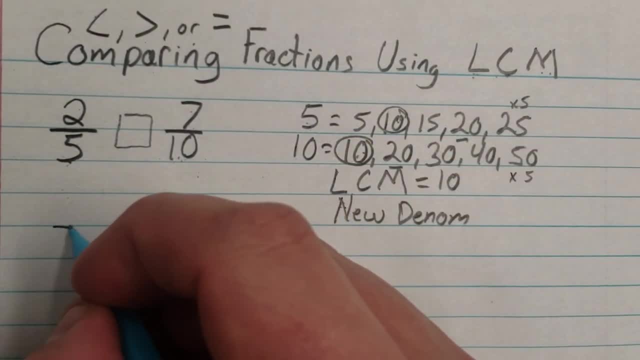 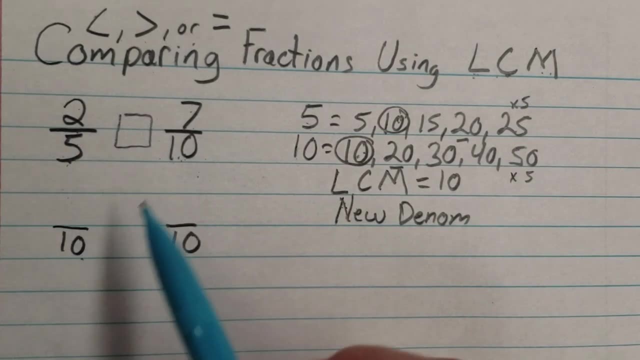 So now we need to make it our new bottom number, our new denominator. What we're going to do is we're going to use our old fractions, the original ones from the question, to make new ones. They're going to have the same value. 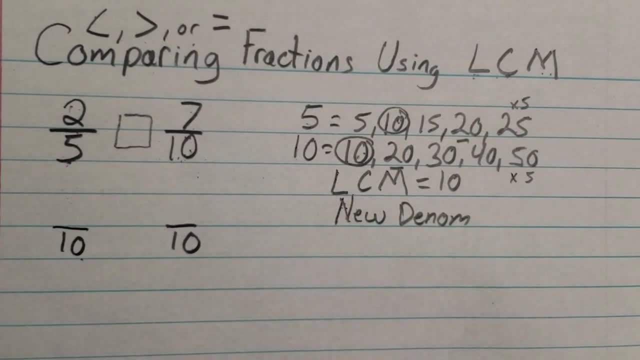 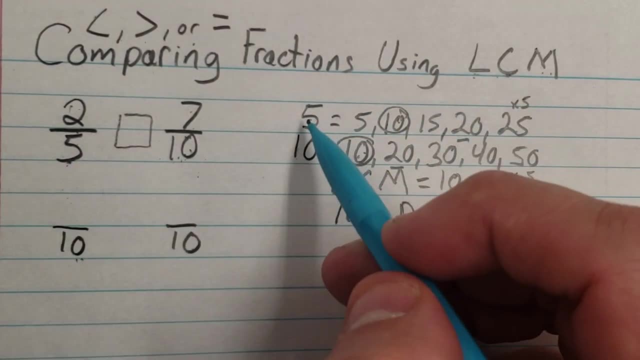 Because whatever we do to the bottom number, we're going to do the same thing to the top. In order to find how we got our new fractions, we just need to look at our LCM. How did 5 get to 10?? 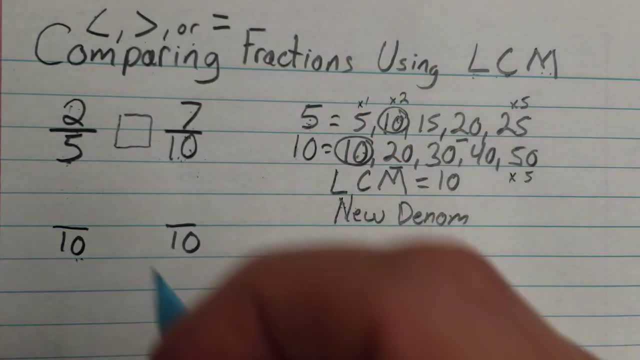 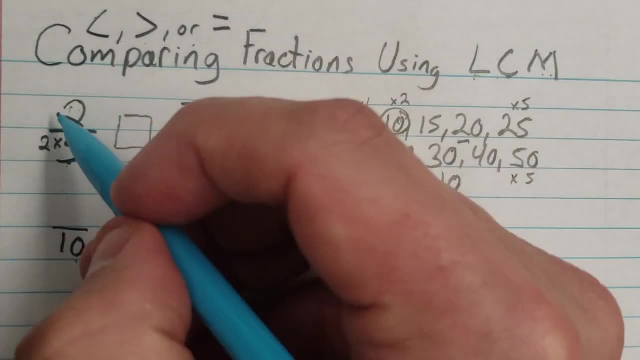 Not times 1, but times 2.. So if you multiply the bottom number times 2,, you get 10.. Whatever you do to the bottom, do the same thing to the top: 5 times 2 is 10, and 2 times 2 gives us 4..